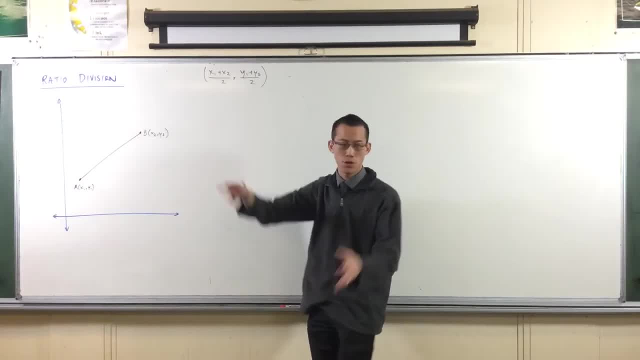 combining them in some way, and then you're dividing through. right, Because if you just add them you're going to be somewhere far away. okay, But if you divide you'll get an average. Now, if I wanted to divide by some other kind of ratio, 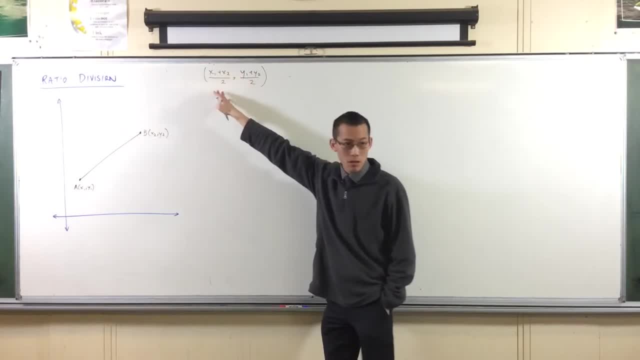 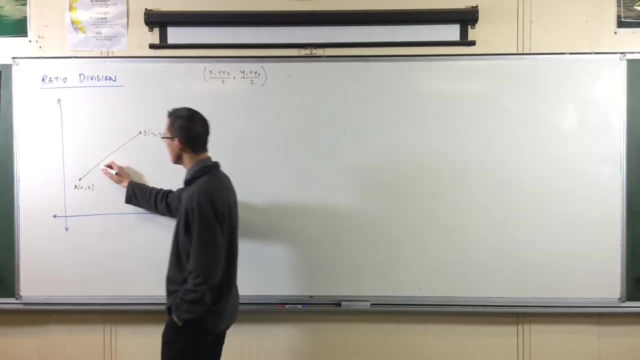 I'm still going to combine the x values in some way, divide through them in some way, and the y values are exactly the same. okay, So to look at exactly how we do it, let's pick a point. Okay, let's call it. 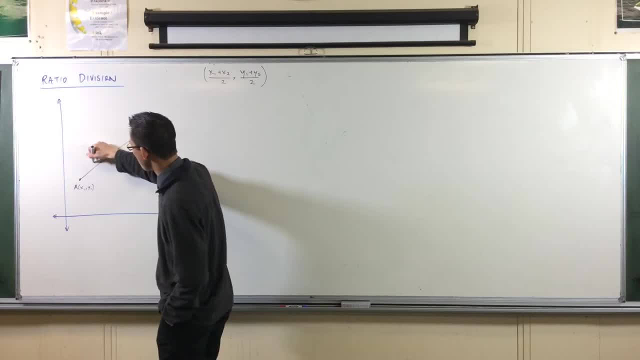 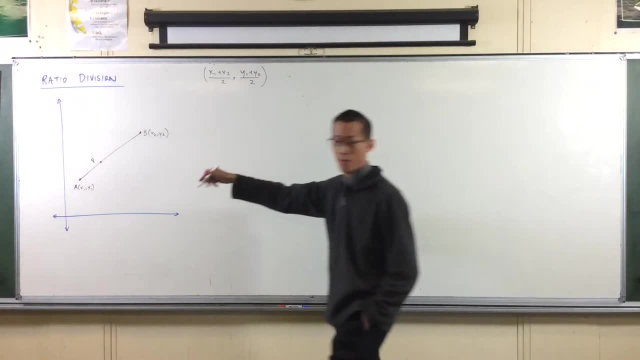 I'll label it up here. actually, Let's call it P right Now, P for point, and I want to know what the coordinates of this thing are, right? This is what I'm trying to find out. So, therefore, I'm going to call the coordinates of this point x, y. 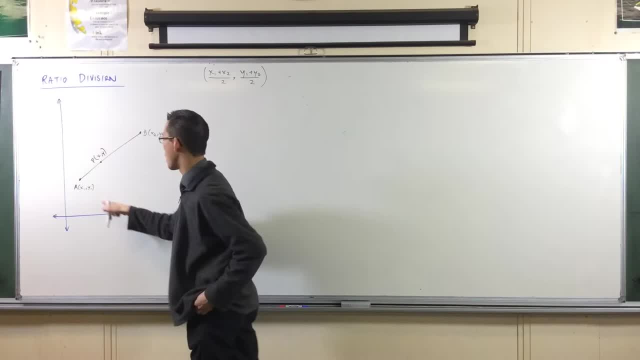 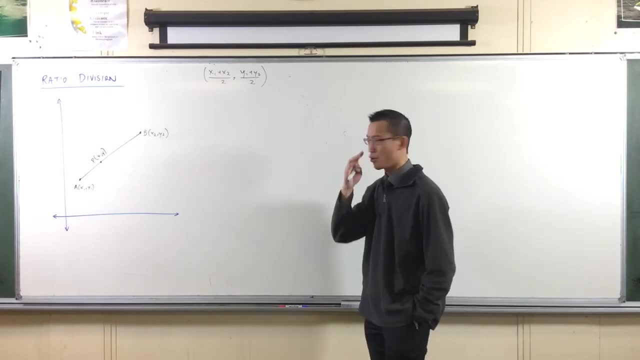 They're the unknowns, Not to be confused with the x1, y1, and x2, y2. that are some numbers you'll be given, okay. So if we're dividing this in a ratio, we need to know what the ratio is right. 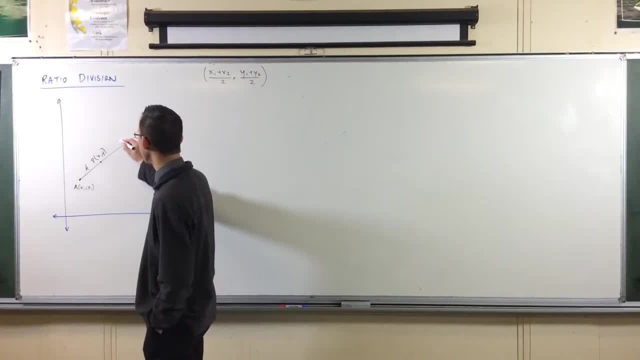 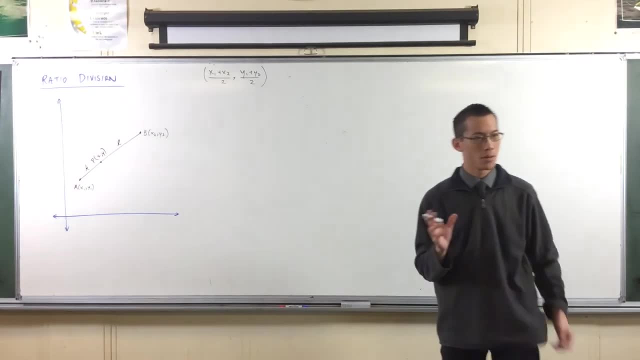 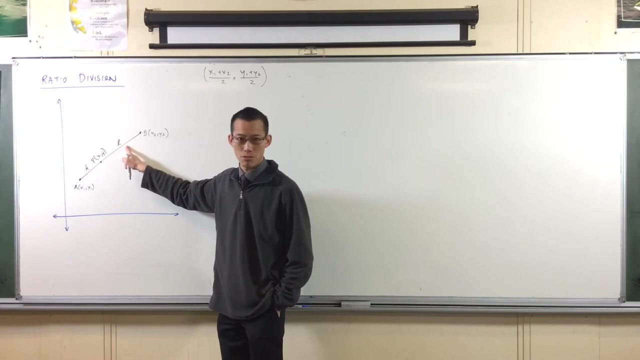 Now, by convention, we're using- We're going to use the letters k and l. Please note: unlike in many other places, here in quantum geometry, order, as you can imagine, is drastically important. Order makes all the difference If, for instance, this was 1 to 2,, 1 to 2,. 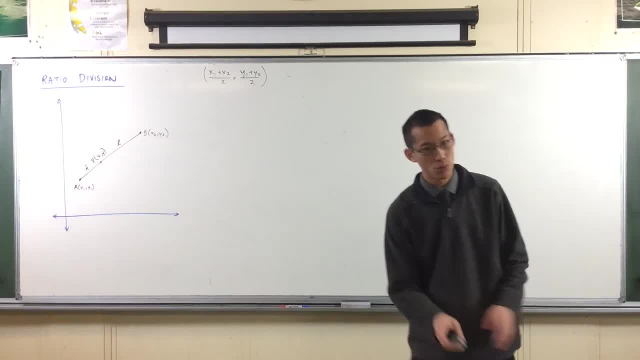 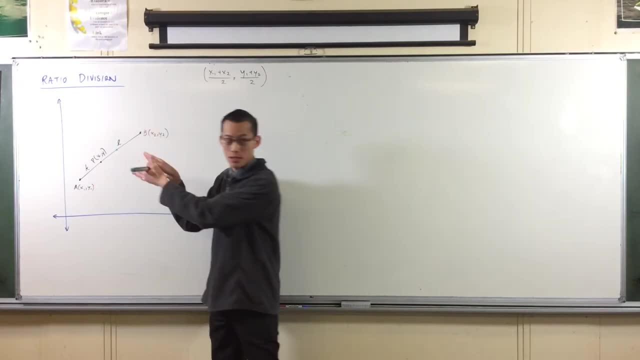 it doesn't take much to see that if I did it in the ratio 2 to 1, I'd be somewhere else, right? Because I'd be going the further distance and then the shorter distance. So 1 to 2 and 2 to 1 are not the same. 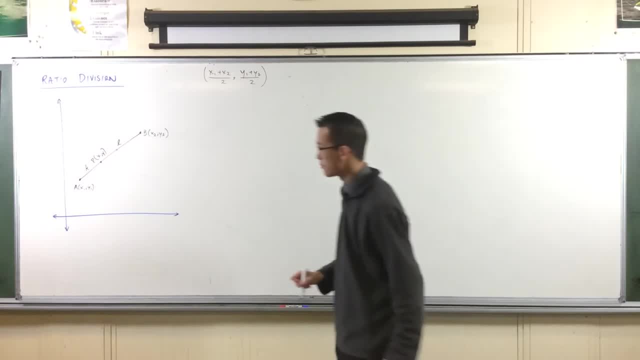 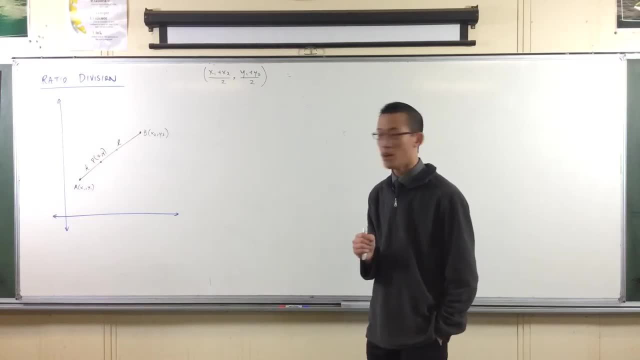 k to l. that's an alphabetical order, and the points that are given to you, a and b, will also be given to you in the order that they want you to divide in, okay? So, for example, here might be a question. 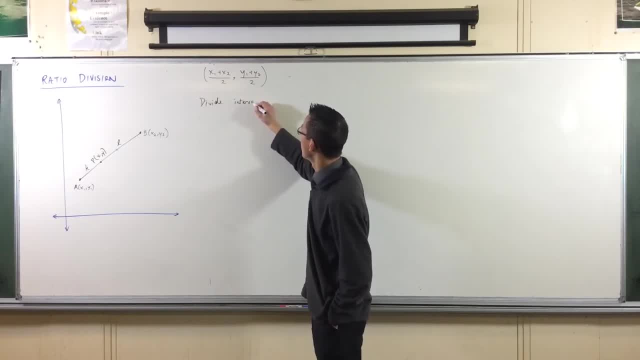 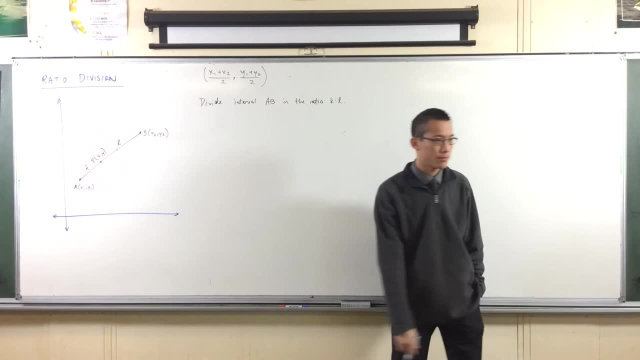 Divide interval a- b in the ratio k to l right Now. in this case it means you're starting with a going to b and you're going to do the k-partial right. So, for example, here you start at a going to b. 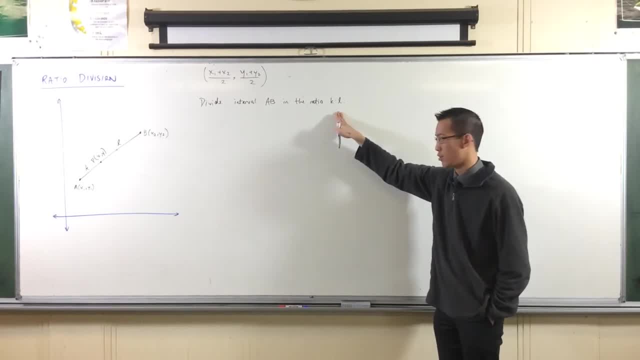 and you're going to do the k-partial, right, and you're going to do the k-partial and you're going to do the k-partial portion first and then the L portion, just like I've shown on my diagram. okay, 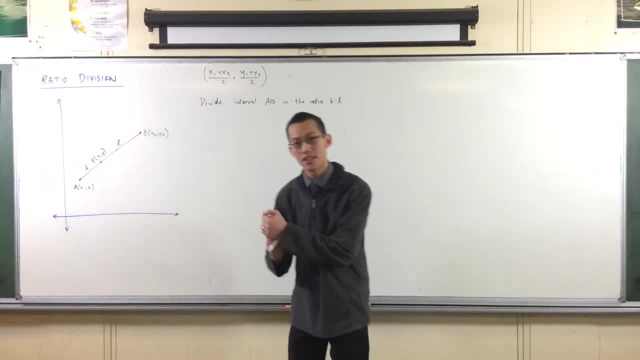 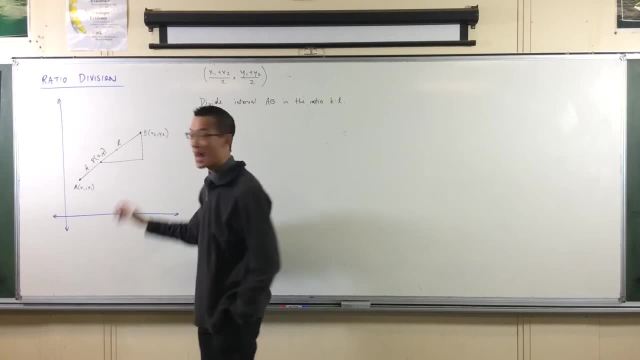 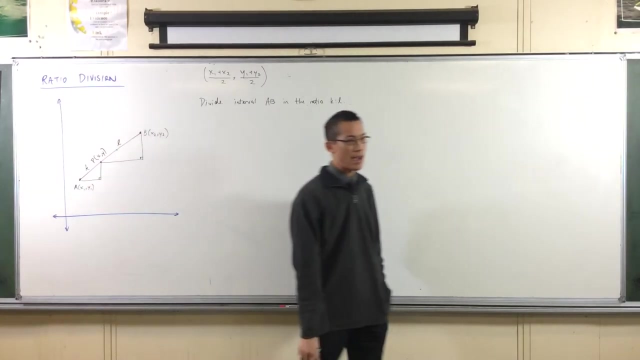 so how are we going to do this? and we're going to take advantage of similar triangles, and so we're going to draw some triangles on here. if I draw down a vertical line, as if I were working out the gradient, and do the same thing, I now have a pair of right angled triangles. okay, because these lines are. 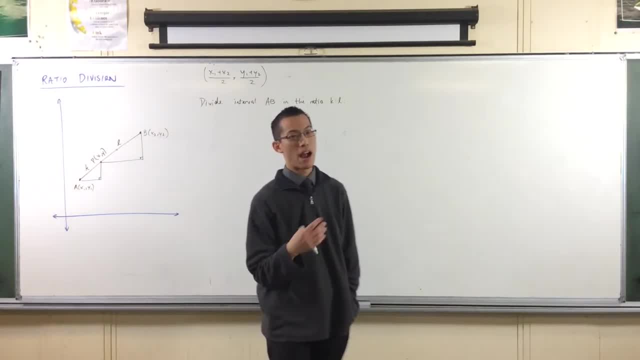 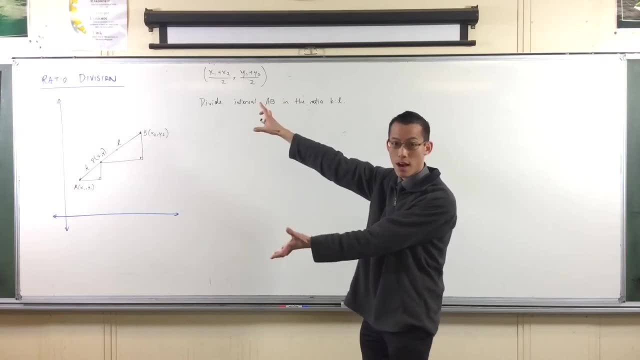 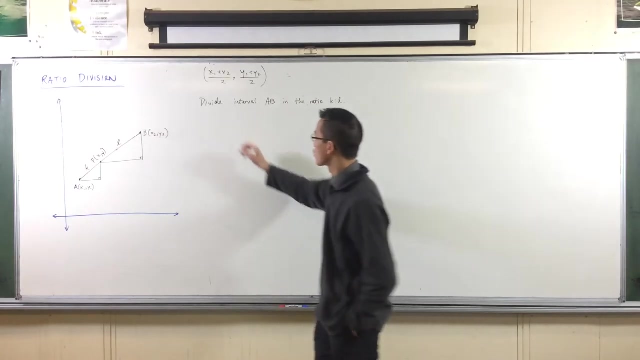 perpendicular. we've got verticals and we've got horizontals. I also have some parallel lines and I have a transversal, namely a- B, so I've got corresponding angles equal, and so on. so these two triangles are similar. that makes sense. we don't need to prove that. we're just using that fact being that triangle. now, 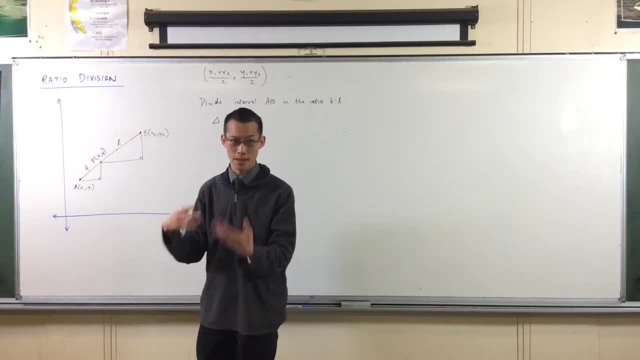 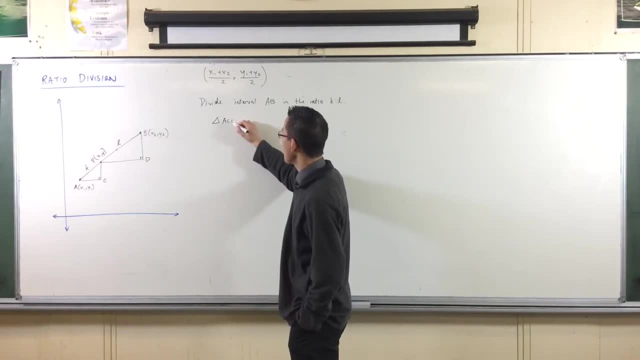 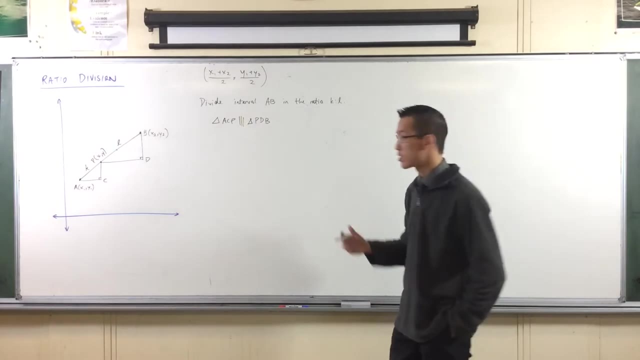 we need some more names here. I've got a, P and B, but to be able to talk about the triangles and call this C and D over here, triangles ACP and triangle P and D B are similar. if we wanted to prove it, the reason would be that they're. 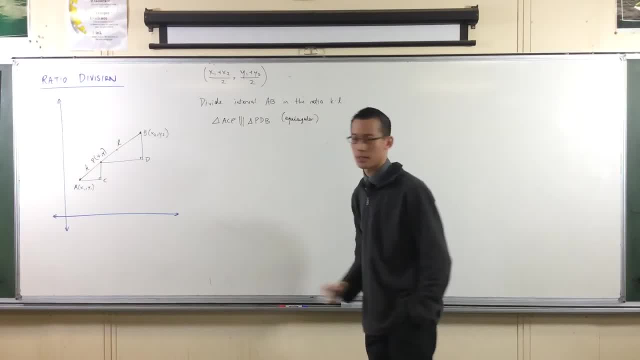 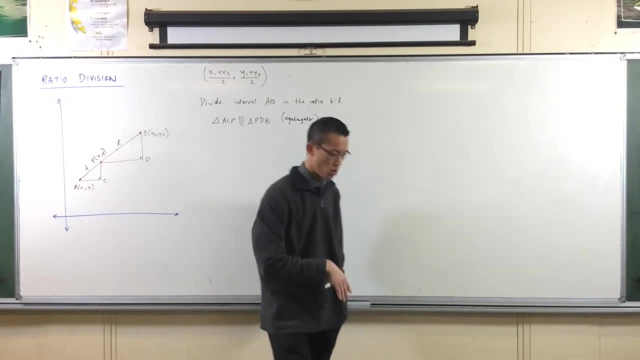 equi-angular. now I'm going to use this to take advantage of. well, I want to work out the X's, and then I want to work out the Y's. okay, so what relationships do I see between the X's and the Y's in this diagram? right, I can see that, for instance, 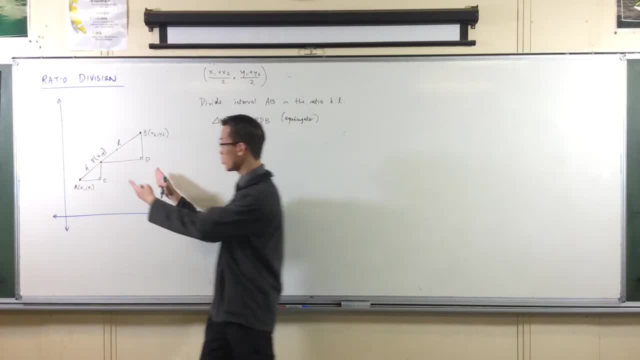 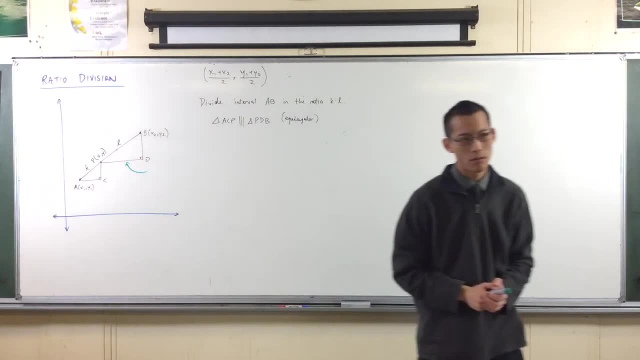 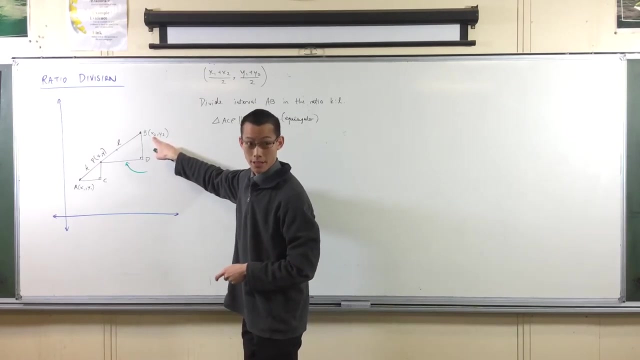 this length here? PD, right? if I just wanted to work out what this horizontal length was, it's just on the X values, right? so how would I calculator? yeah, yeah, yeah, good. so x2 is how far I am away from the axis right and X is how. 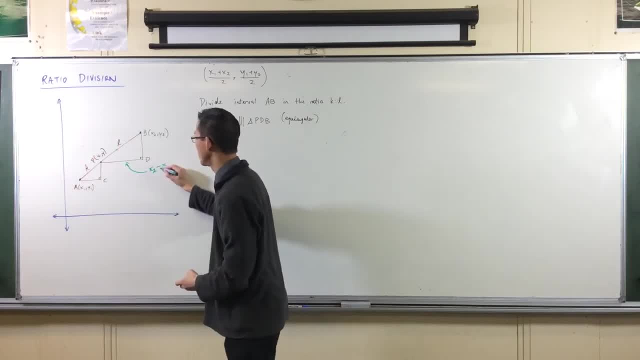 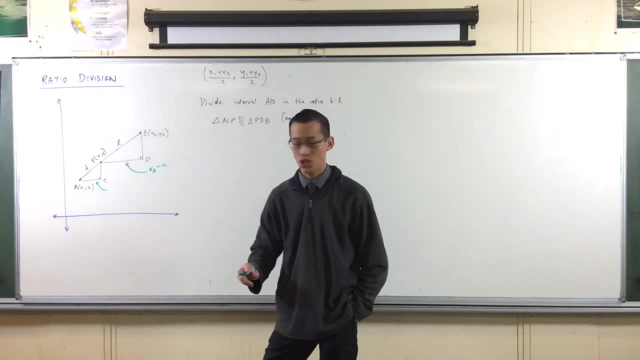 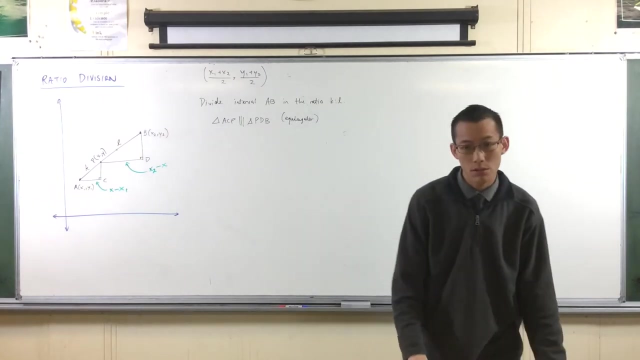 far. this is away from the axis. so this will be the difference: x2 minus X, that's PD. but is the exactly the same logic? I can get a C right, which is side from X, and I'm taking from excel, taking away x1. So I have those two distances, so now I can compare different sides to each. 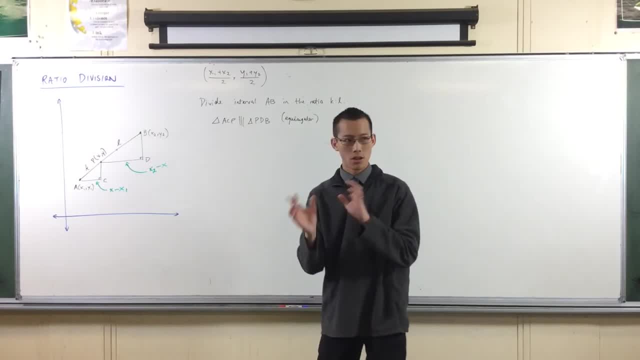 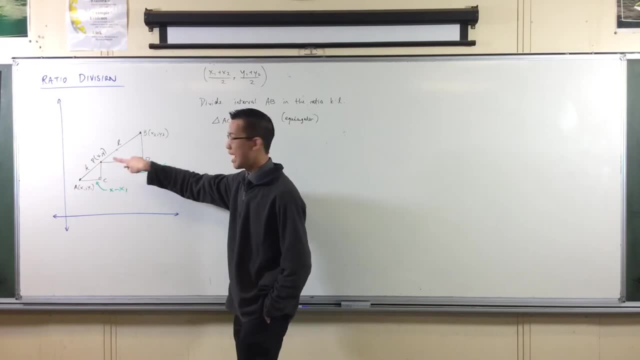 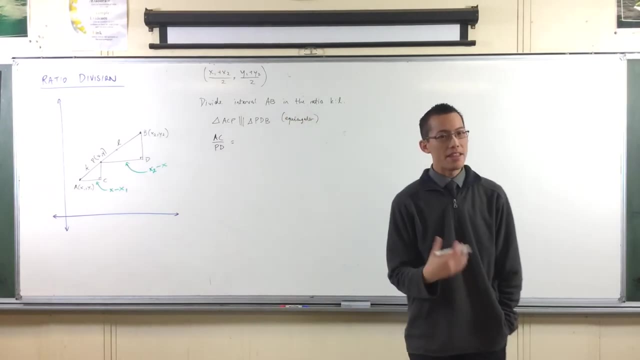 other and they're all ratios. So I can say corresponding sides and similar triangles are in the same ratio. So the corresponding sides might be, say, AC and PD. They're corresponding sides, aren't they? So I can say AC on PD and the other pair of corresponding sides. 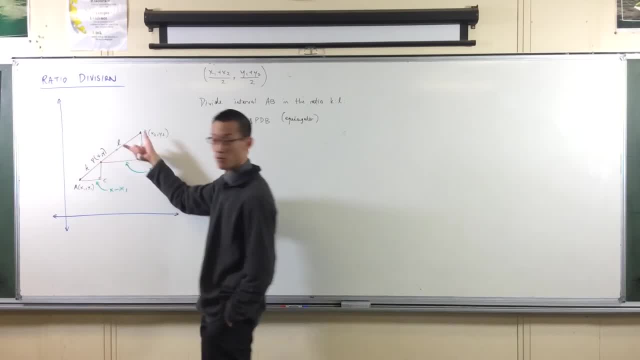 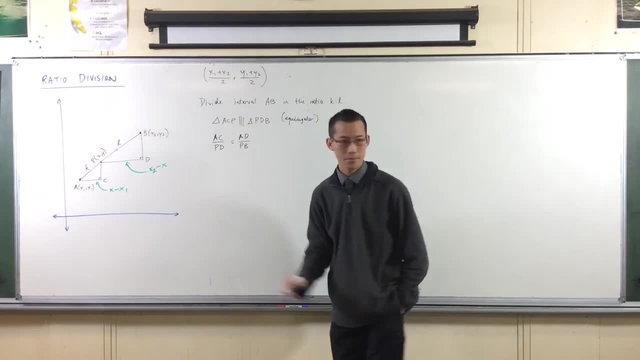 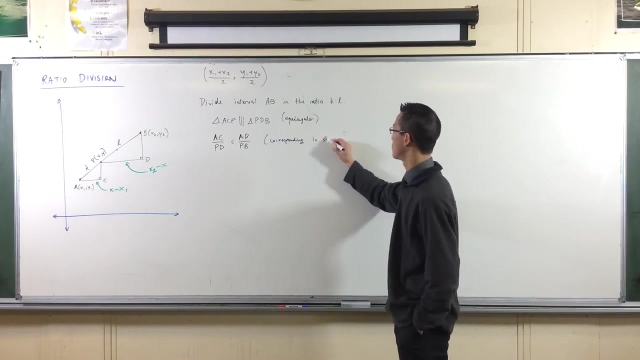 the ones that I know something about are the ones that I've been given ratios for, So they're going to be AP and PB, And the reason why, corresponding sides and similar triangles. Okay, now, conceptually, that's all there is to it. 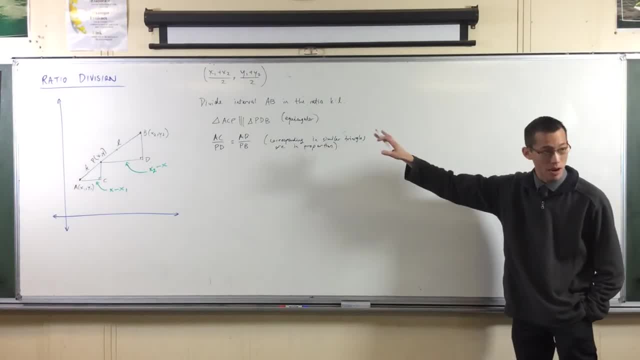 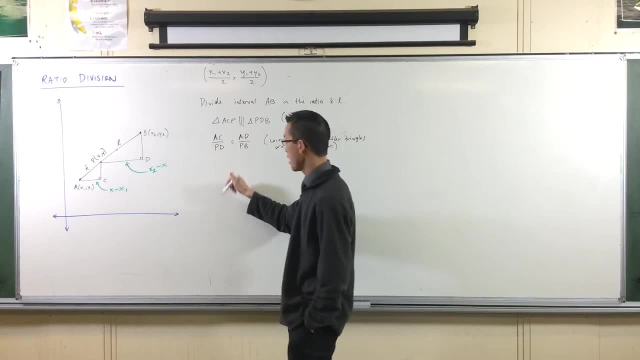 Just a little bit more information. Okay now, conceptually, that's all there is to it, Just recognizing that similar triangles, relationship and picking out the right sides From here. let's just do our substitution. We've already noticed in green what AC and PD are. AC is: 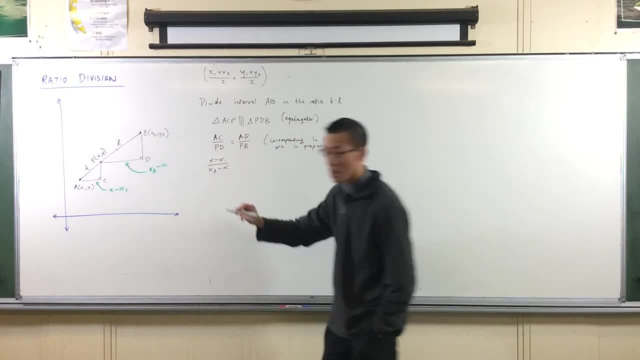 going to be this and PD is going to be that. By definition, these two, these hypotenuses, they're the sides that are in ratio. So I've got K first and then L, And all I want to do here is I'm trying to find this thing right, Except I know it's something different. I 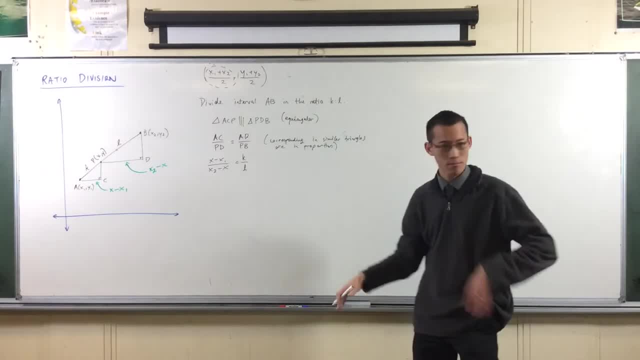 have to make X the subject. You see that? Okay, so let's just rearrange this. go through motions, It's not hard right? Okay so let's just rearrange this. go through motions, It's not hard right. 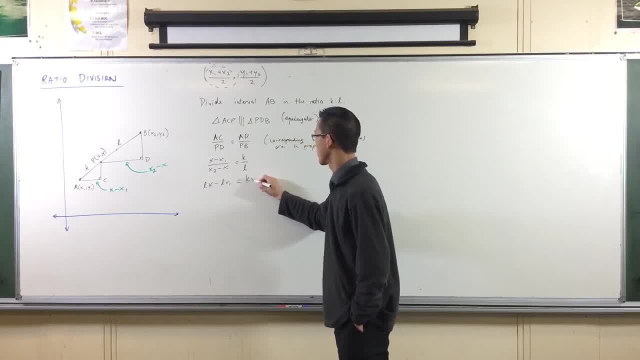 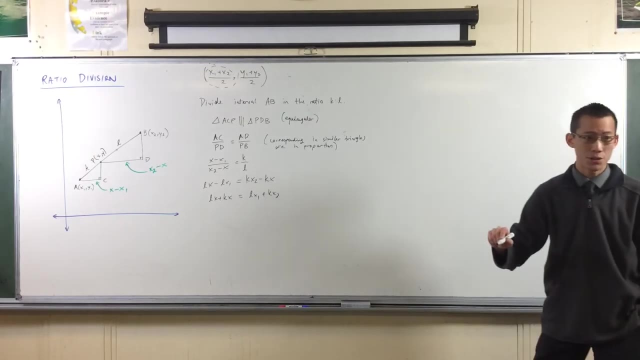 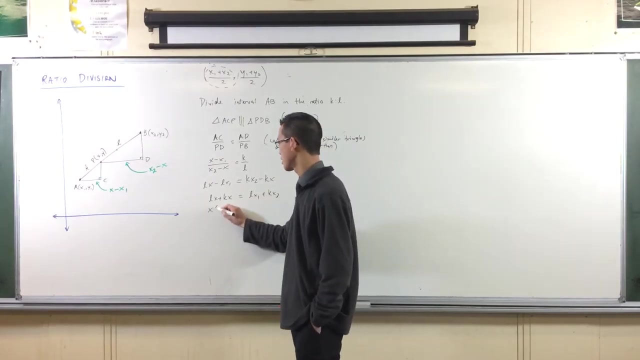 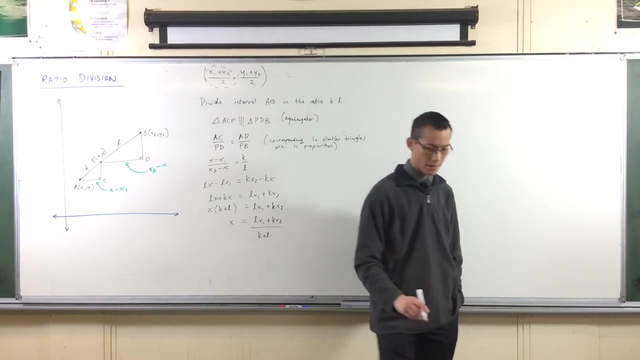 You covered that I've just cross-multiplied and expanded out. Here I'm going to make X the subject. Here I'm going to make X the subject, which will give me k plus l, and then I'll divide through. okay, now there are a couple of things to notice. 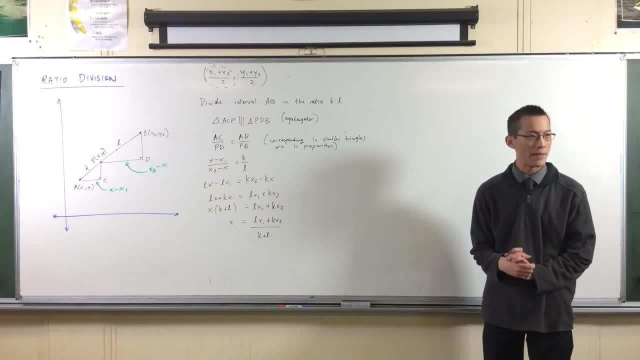 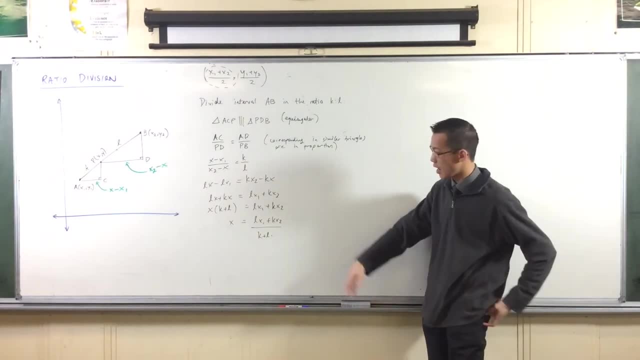 number one. I don't need to go through this whole process again for the y values. it will play out exactly the same, but with y's instead of x's. so I can just use this and say similarly: my y corner will be ly1 plus ky2 on k plus l. 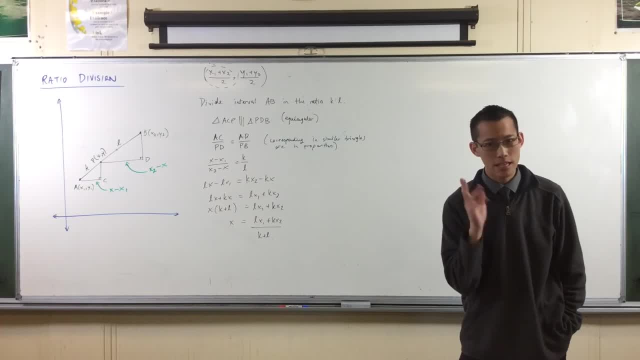 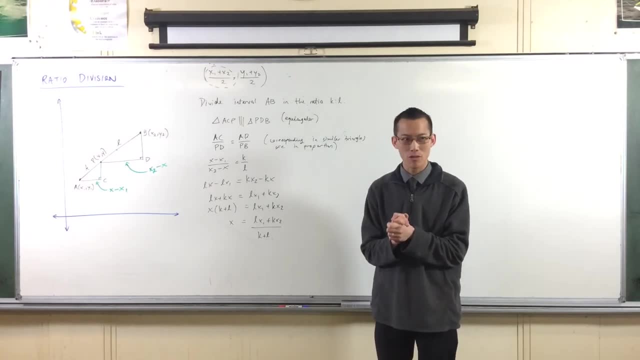 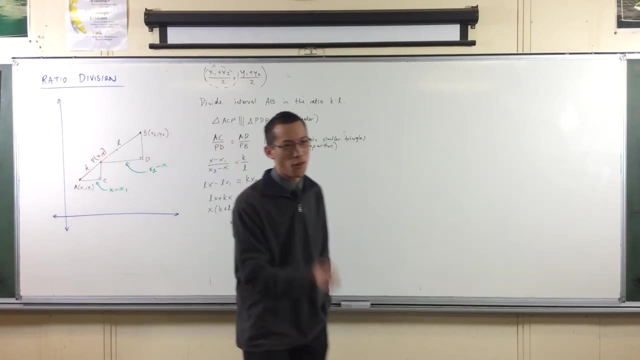 that will still be the same. secondly, please note- and this is what is drastically confusing for the bill- alphabetically which one comes first, which part of the ratio comes first. alphabetically, k comes first and then l, but in the formula, in the formula, they're mismatched.